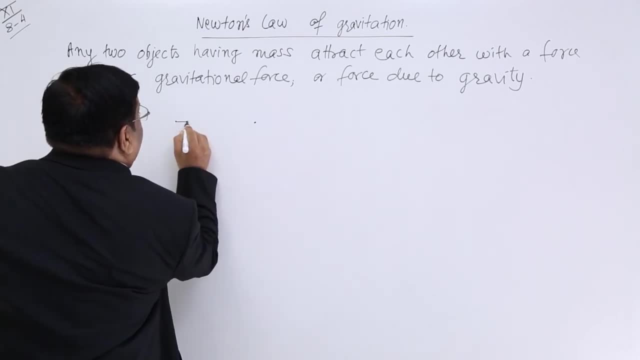 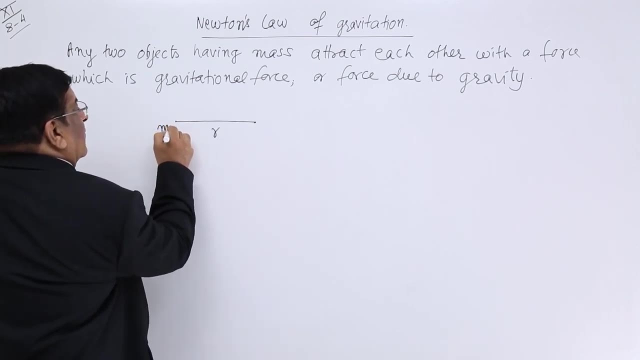 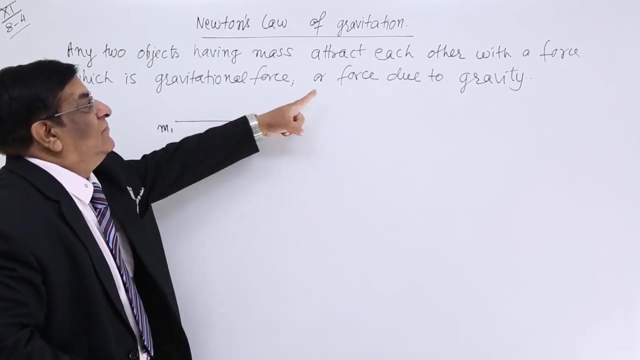 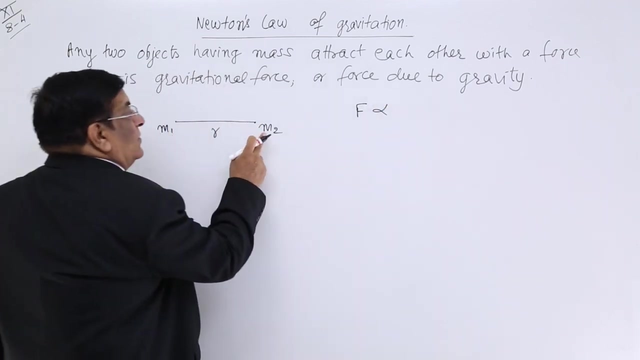 These two point masses which are located from each other at particular distance, At any distance, are: one point mass has mass m1 and the other has got mass m2. Then they will attract each other with force due to gravity or gravitational force. This force is proportionate to both the masses. 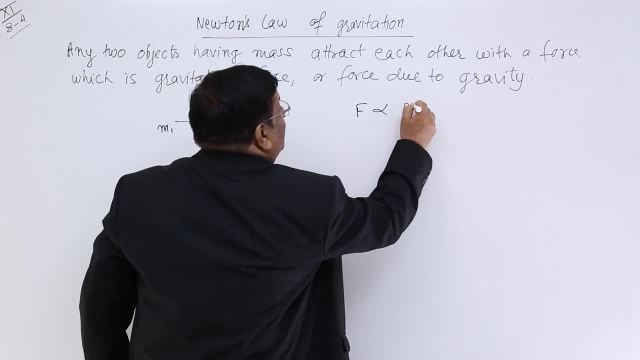 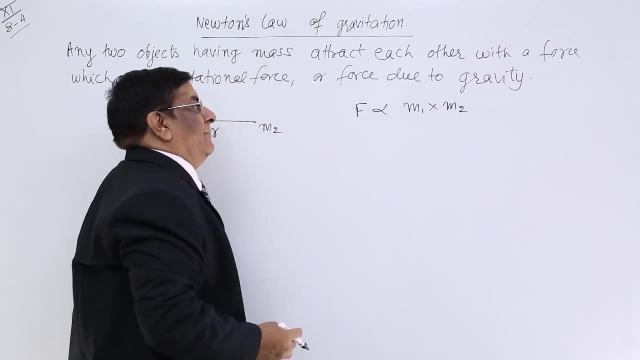 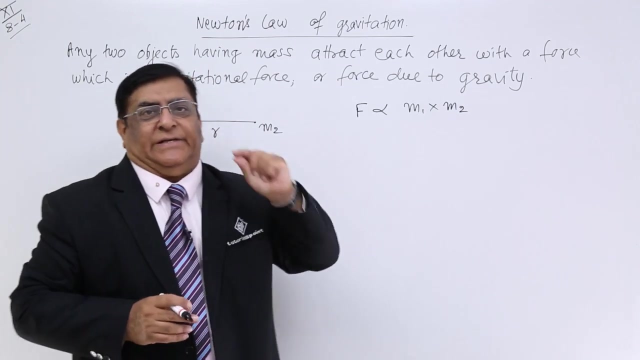 And how do we have to take the masses? That will be multiplicity, Multiplication of both the masses. So the force is proportionate to the product of m1 and m2.. This is the one thing. Second thing: he said that when the distance increases, the force decreases. It decreases rapidly. 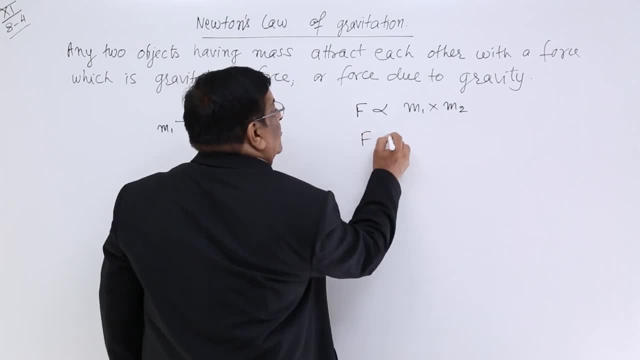 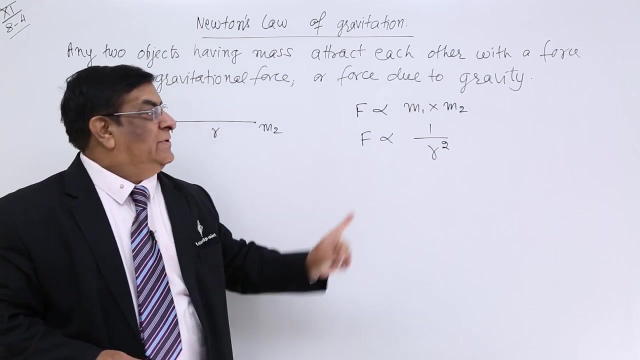 And for that he decided, he told us that force is proportionate to inverse of square. This is a very important thing: Square of the distance, It may not be power of mass, It may not be power of 1.. It may not be power of 3,, power of 7,, power of 8.. This is power of 2.. 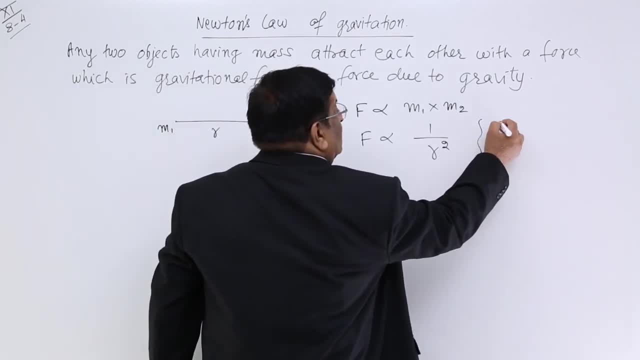 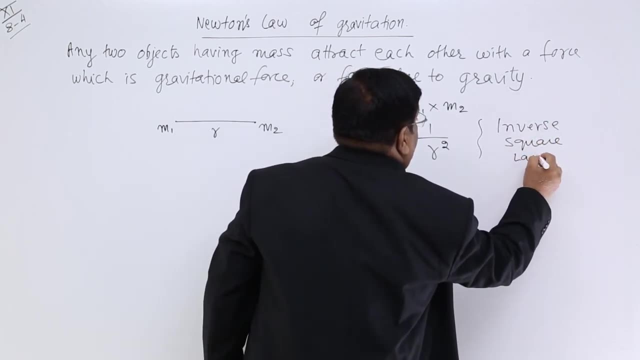 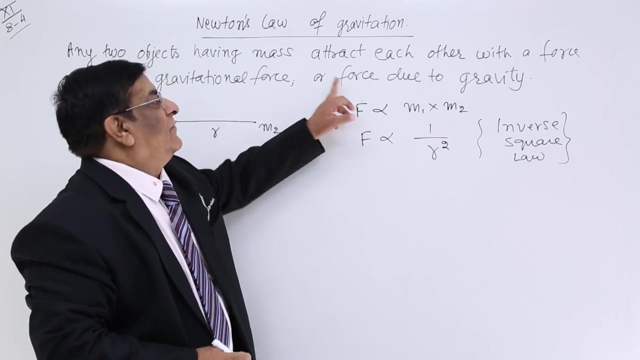 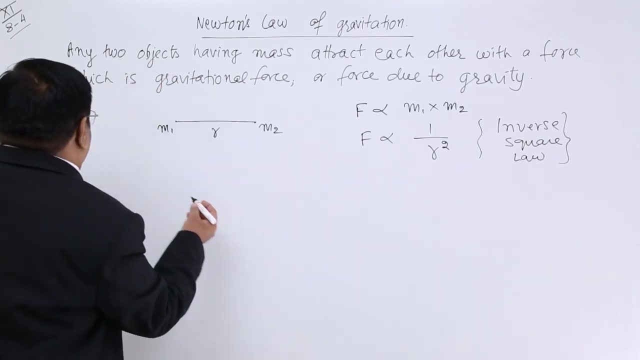 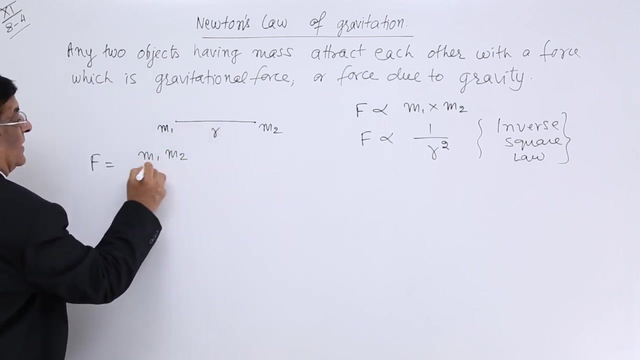 This Because this is power of 2, this is known as inverse square law. So he said that this is the laws of the force of gravitation between the two masses. Now, if an equation is to be made, then he made the equation that force is equal to m1, m2 upon r square. and for this equal, there has to be one constant of equality. 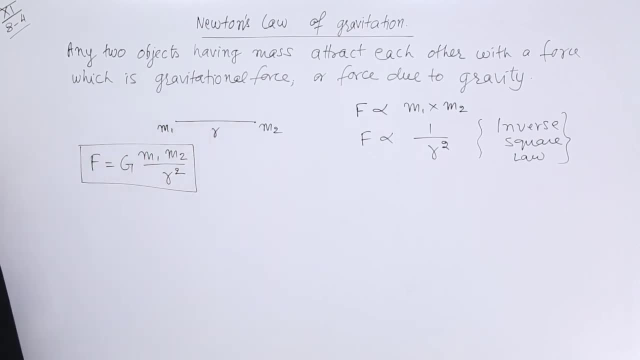 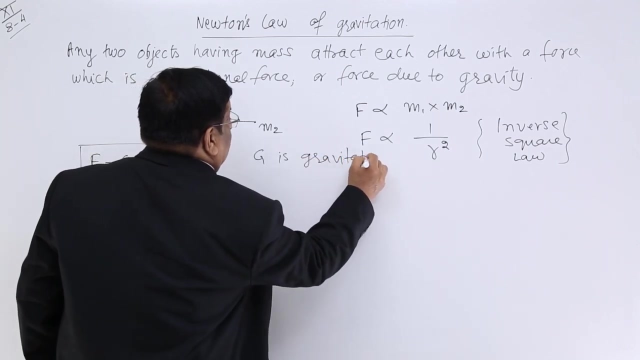 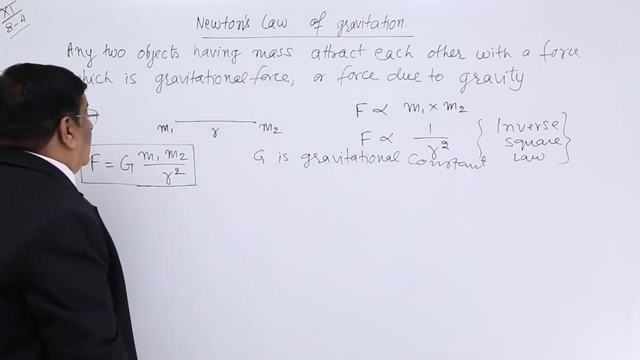 And he put this gravitational constant, G, Capital G, And then he described what is this G and we have to study about it. G is gravitational constant. G is gravitational constant. Now, this is between the two masses and the distance is r. 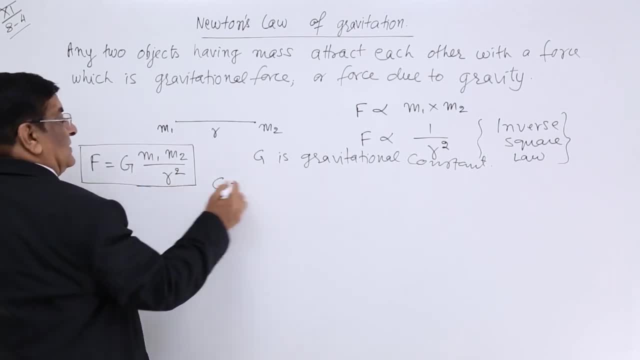 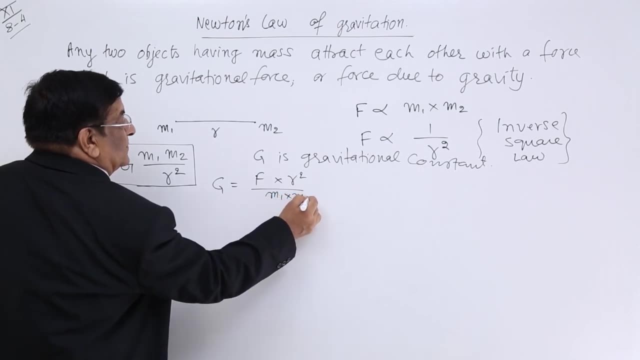 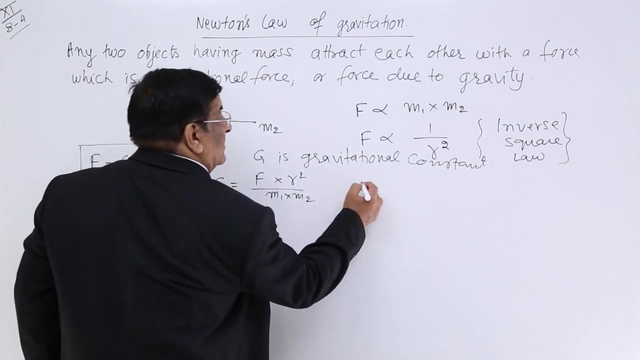 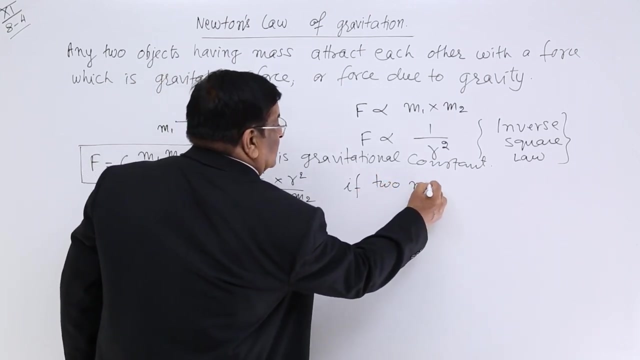 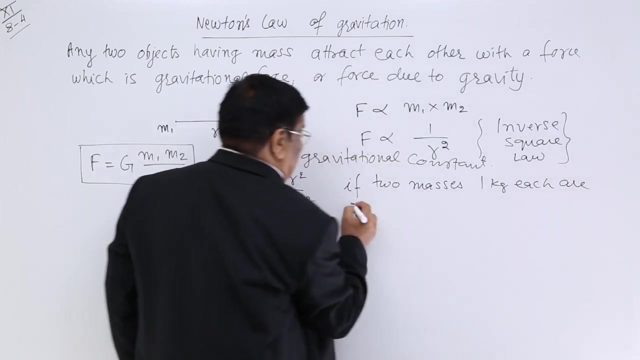 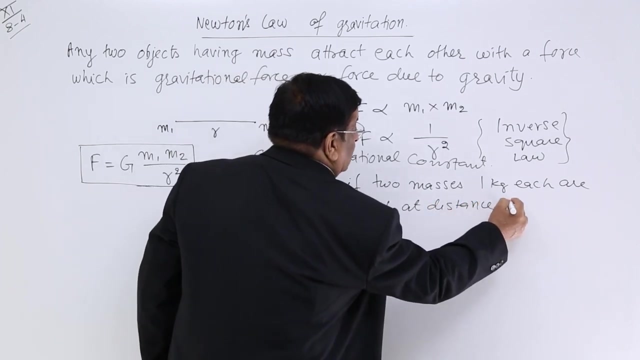 So can we find out G? G is force multiplied by r square upon m1, m2.. With this we can define G, That G if two masses of 1 kg each, If two masses 1 kg each are placed at distance 1 meter. 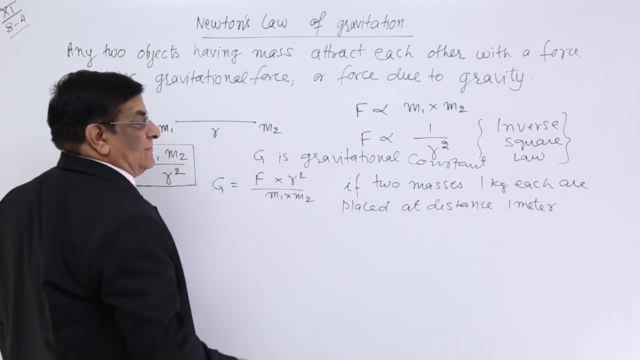 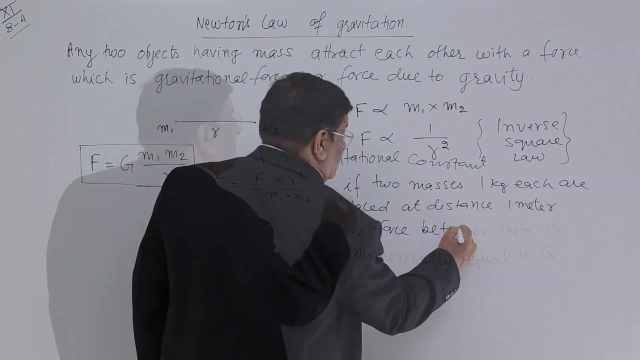 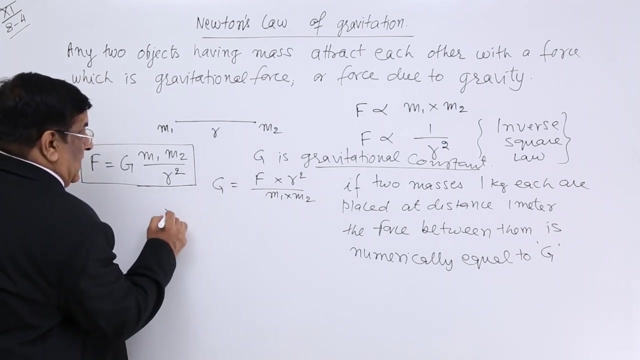 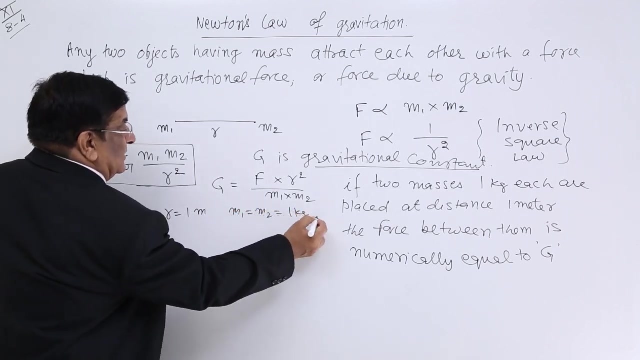 1 kg. 1 kg 1 meter. Then force between them is equal to G, Gravitational constant r is equal to 1 meter, m1 is equal to m2 is equal to 1 kg. Then we get this definition. 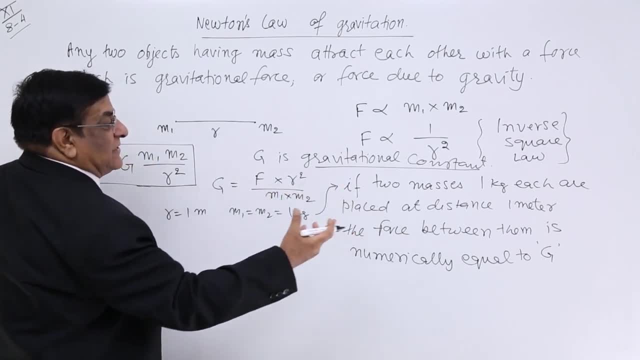 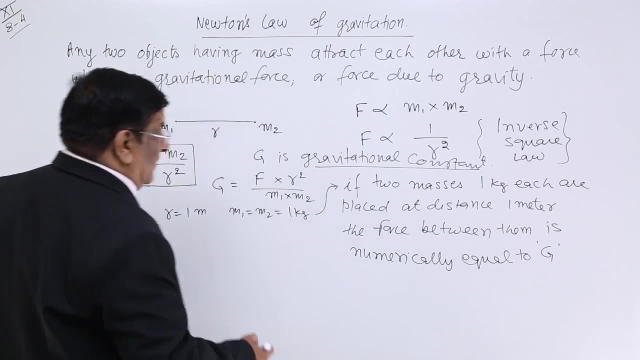 And this we have done Practically. when it was done, we got certain value of G and certain unit of G. The value of G we got is 6.67 into 10 to the power minus 11.. And what should be the unit? 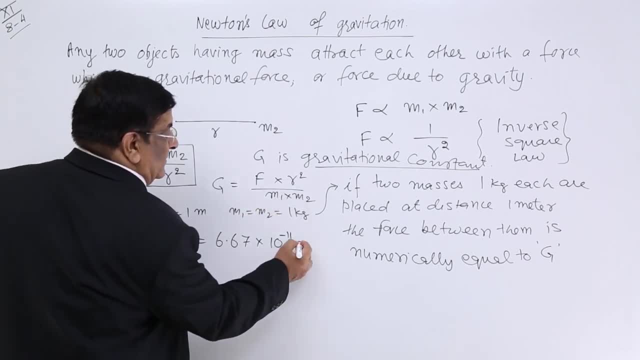 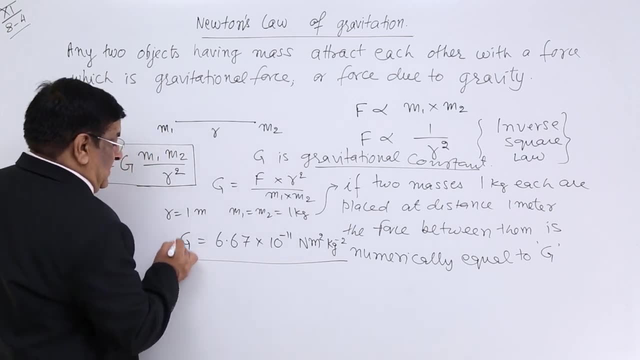 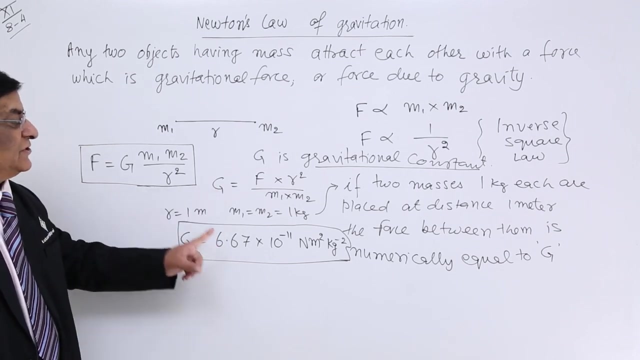 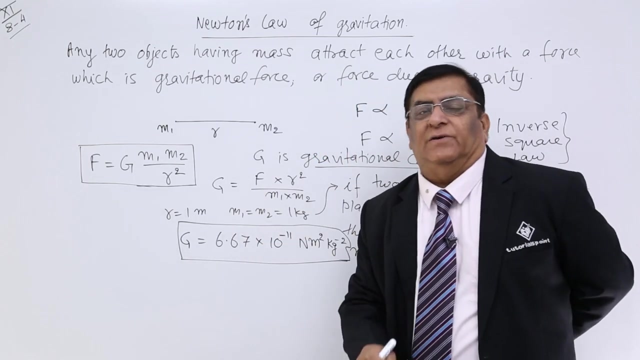 Newton meter square per kg square. Newton meter square per kg square. Please remember this. This is G Gravitational constant, And he said that this G is a constant which is true for earth to sun relation, Sun to the other star's relation. 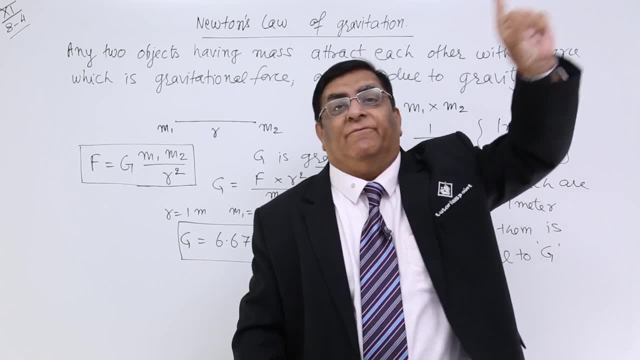 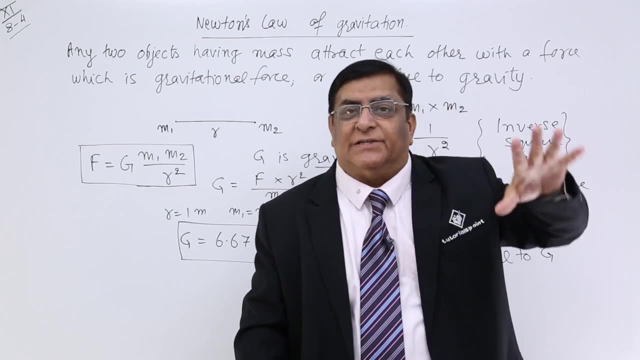 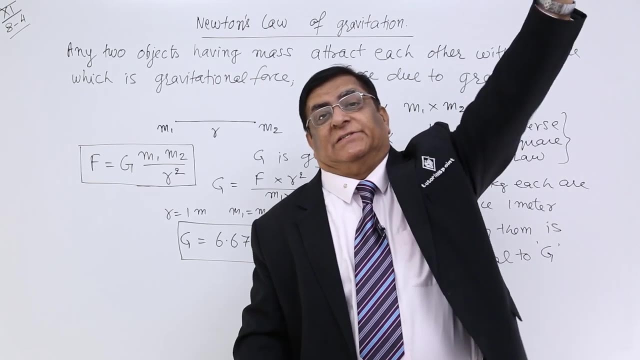 And third star, fourth star: everywhere this G value is same. It is not affected if the stars are changing. It is not affected if the medium is changing And it is not affected whatever is the distance. So it is same all over the universe. 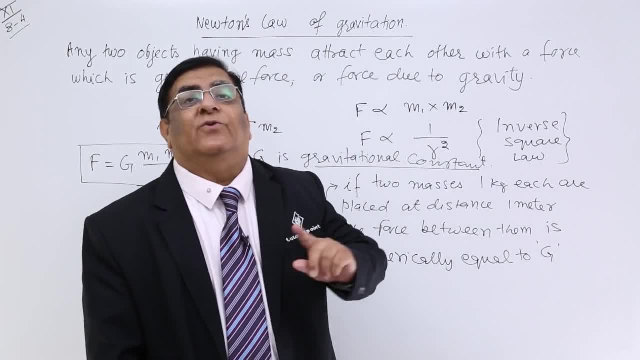 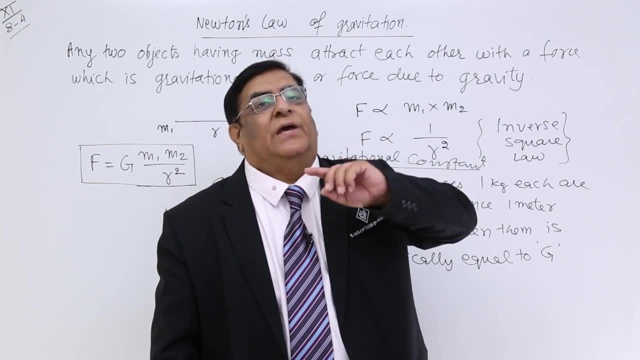 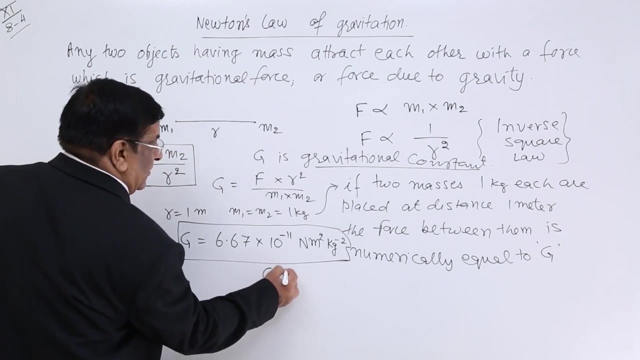 Therefore we give it a title that this is a universal constant. Any constant which is not changed All over the universe and it can be used anywhere in the universe, That is known as universal constant. So G is a universal constant. So what is G? 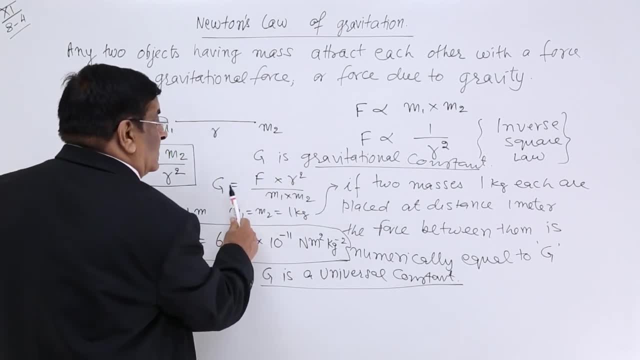 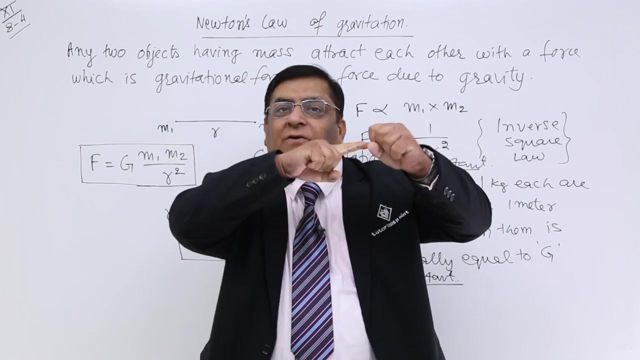 G is gravitational constant, which tells us about the force, The force between two 1 kg objects kept at 1 meter distance. Two 1 kg objects kept at 1 meter distance, Whatever is the force, that is the unit gravitational force given by gravitational constant. 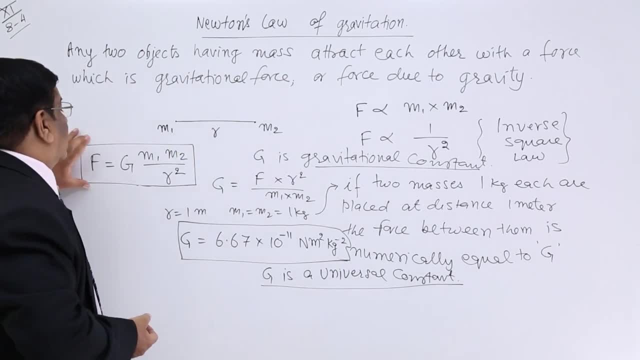 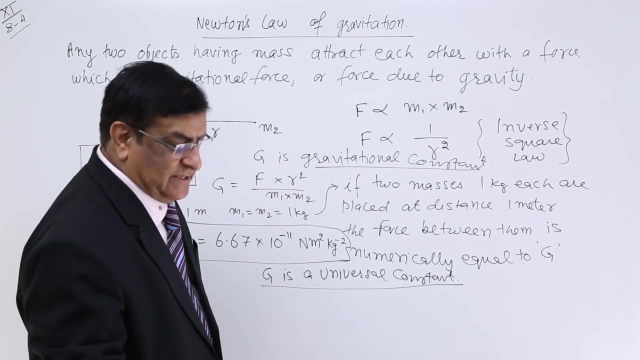 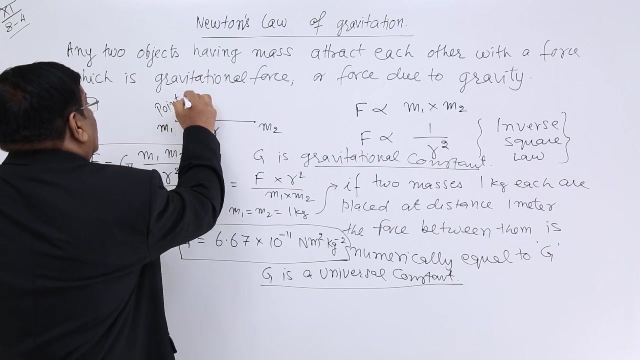 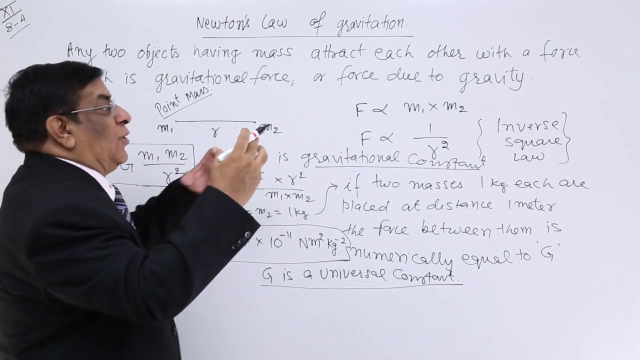 Capital G. So this is Newton's law of gravitation. For the Newton's law, one compulsory thing was that he derived it. he made it for point masses Because he was not sure if this is a big body And other body is very close to it. 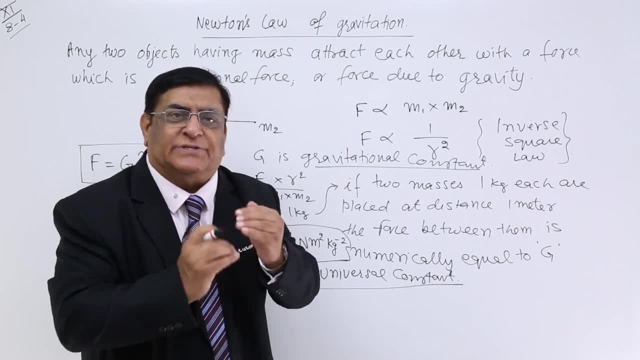 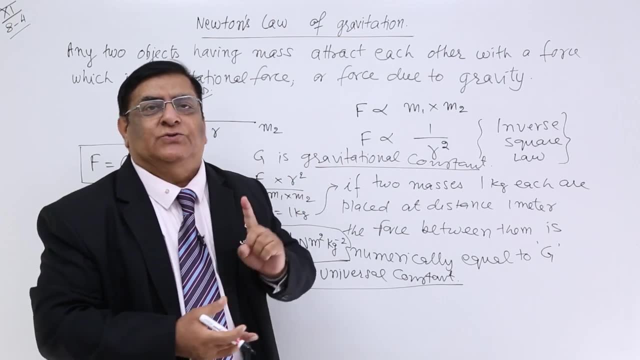 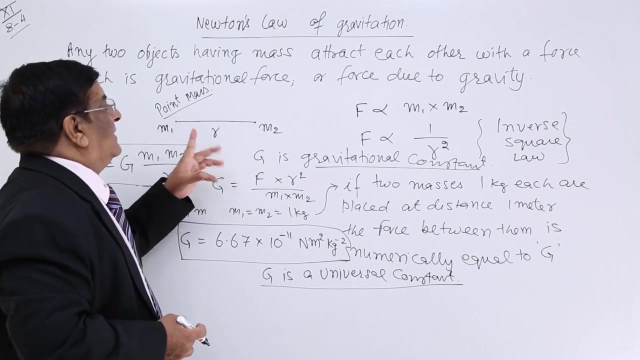 Whether this force will be applicable or not, There has to be certain changes which have to be done According to shape of the system, shape of the body. So this is the basic law between the two point masses kept at a distance: r. 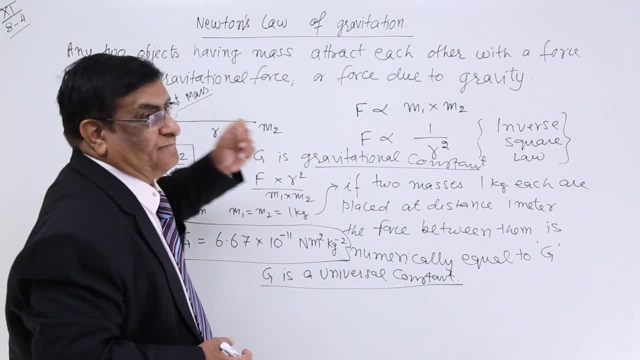 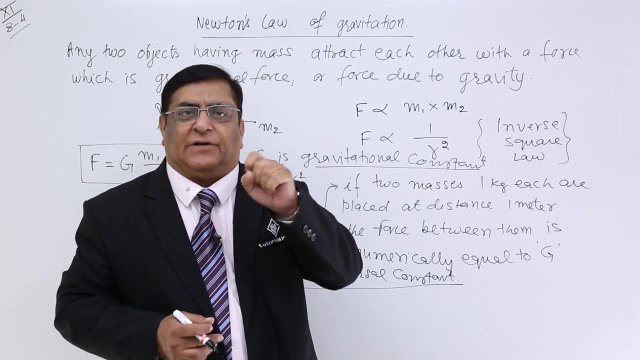 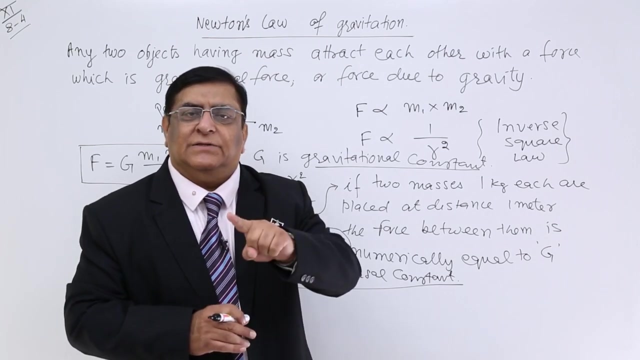 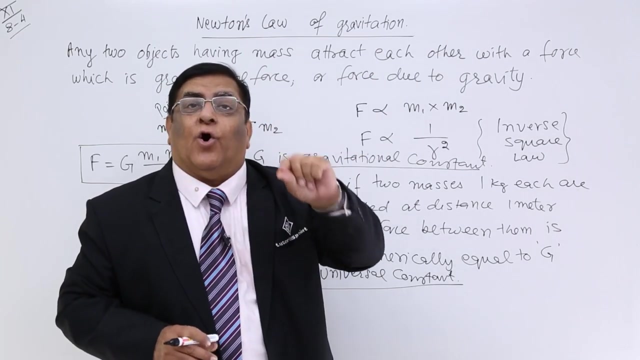 This gravitational force. we know its many properties. It is a force of attraction only. There is no repulsion. Second, it is not affected by medium. Third, it acts for a very long distance, Whatever is the long distance. So it is a long range force. 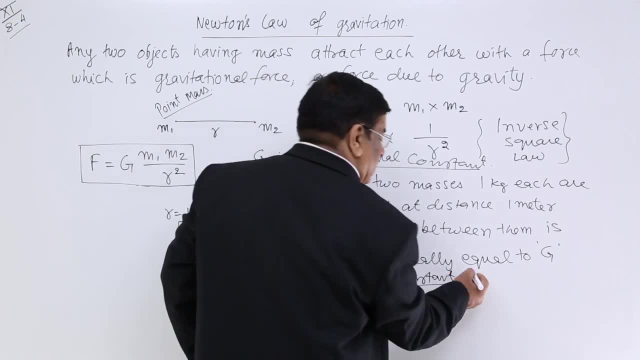 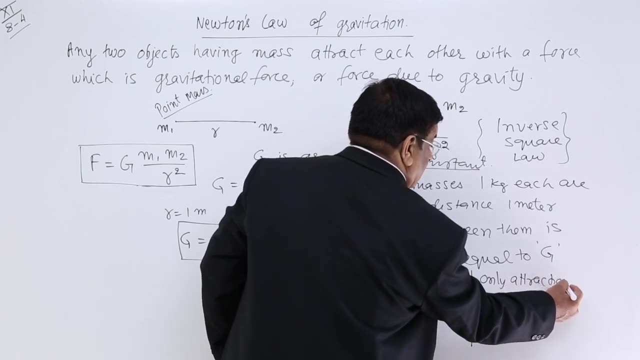 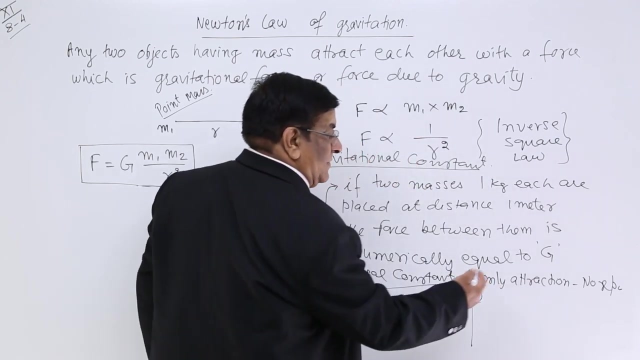 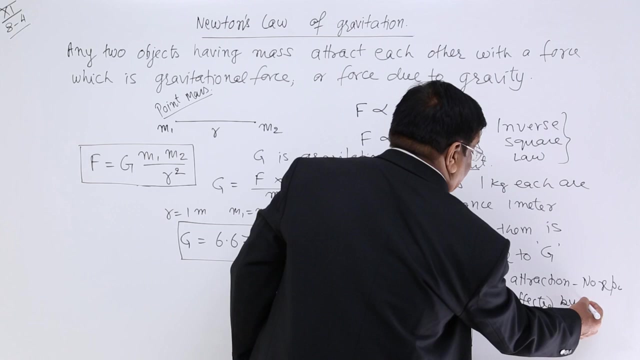 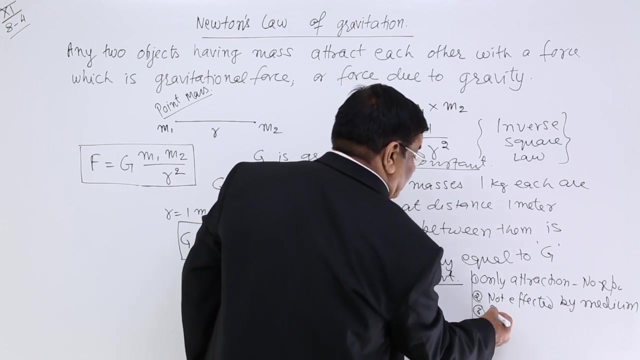 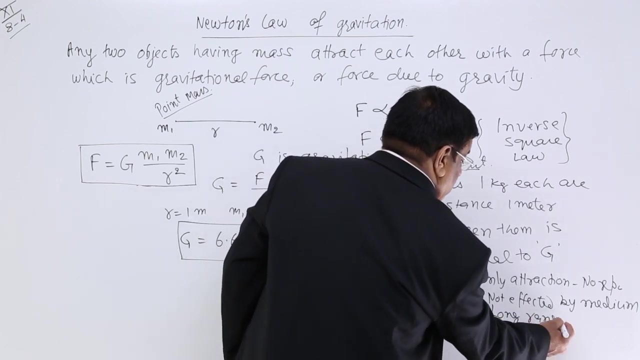 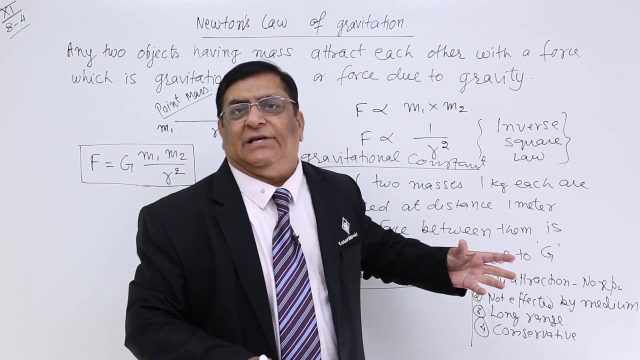 So we can just revise it. Only attraction, No repulsion. Second, not affected by medium. Third, long range. Fourth, conservative. When we were studying work power, energy, I have explained to you what is the meaning of a conservative force. So gravitation is a conservative force, So